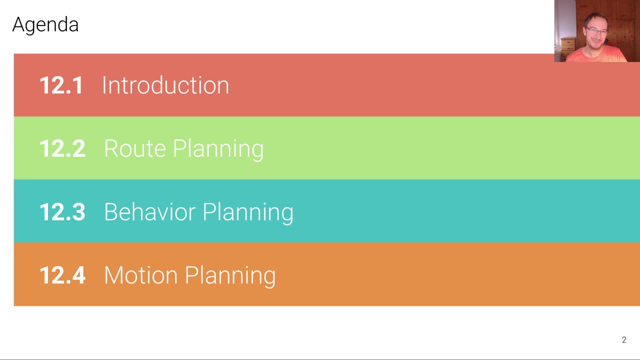 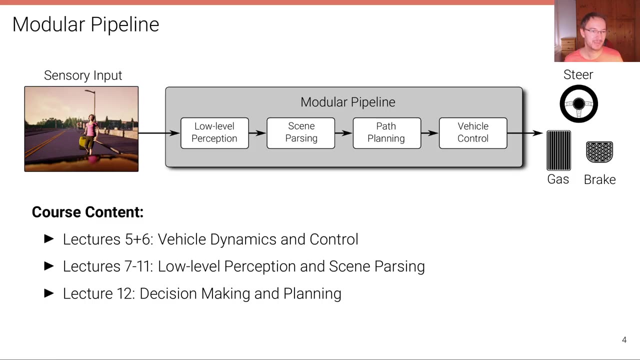 the actual vehicle trajectory that is then fed into the controller for execution. So let's start with the introduction. This is a slide that we have seen before. This is the slide of the very simplistic, simplified modular pipeline, where we have discussed at a very abstract level four different modules: The low-level perception. the low-level perception. 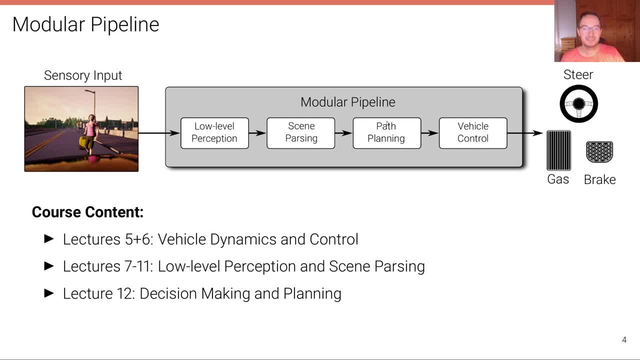 the low-level perception of the different modules and the low-level perception of the different modules, The scene passing module, the path planning module and the vehicle control module In lecture number five and six. we have discussed the vehicle control part In lectures five. 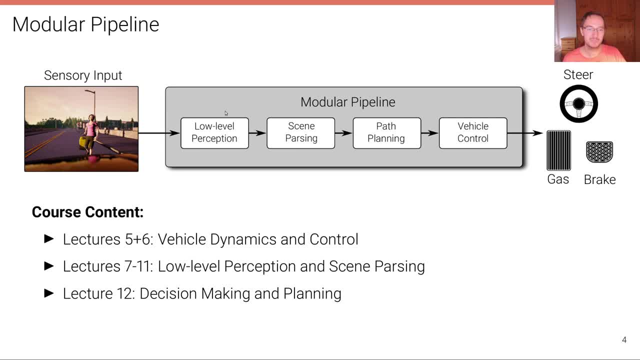 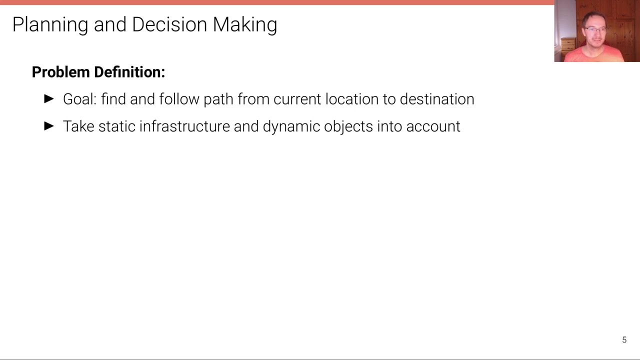 to 11,. we have discussed the low-level perception and scene passing part, And now we're going to discuss the connection from the perception to the control, which is the decision-making and path planning stage. here Let's first define the problem, The goal of the decision-making and path planning stage. 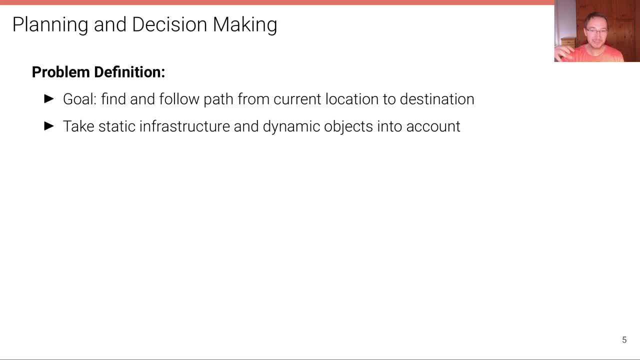 is to find and follow a path from the current location of the vehicle to the destination And, of course, while doing so, we want to take the static infrastructure and dynamic object objects. The input to the decision-making and path planning stage is the vehicle and environment. 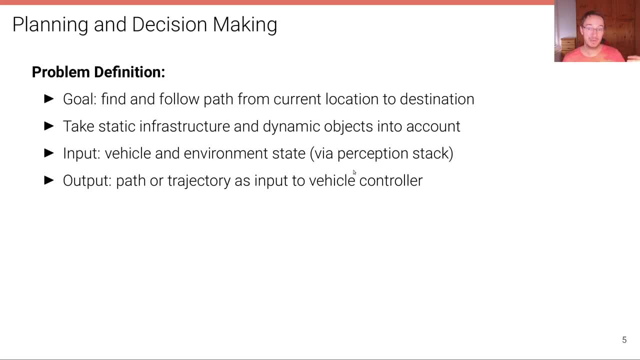 state as perceived through our perception stack, And the output is the path or trajectory as input to the vehicle controller. However, as it turns out, driving situations and behaviors can be very complex And therefore it's difficult to model the entire problem of decision-making and planning. 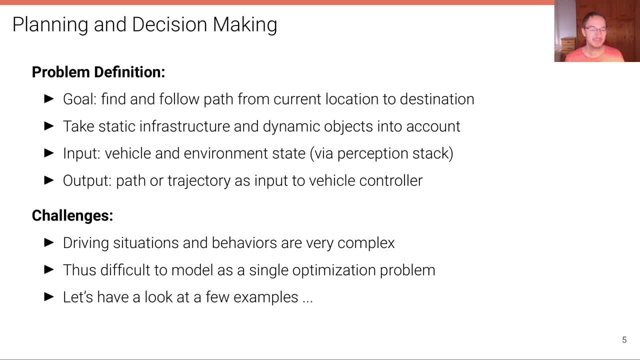 as a single optimization problem, And so what we typically do instead is we decompose this complex task into a hierarchy of simpler sub-problems. But let's first have a look at a few examples of such situations that motivate the need for decomposing this problem into sub-problems. 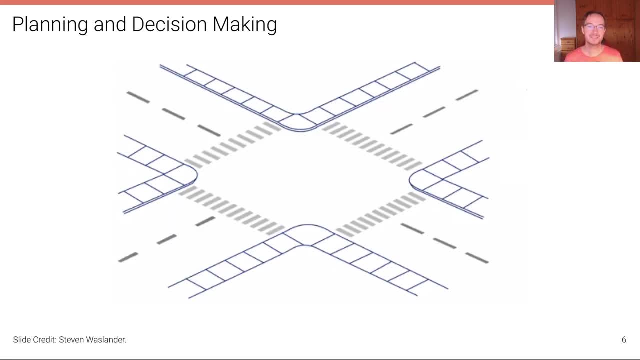 So here's an intersection: What states can a vehicle be in? What situations can a vehicle encounter? Let's suppose this is the vehicle that we consider. One situation the vehicle could be in is just a simple speed tracking task where it tries to follow the lane at a set target speed of 30 miles per hour, say. 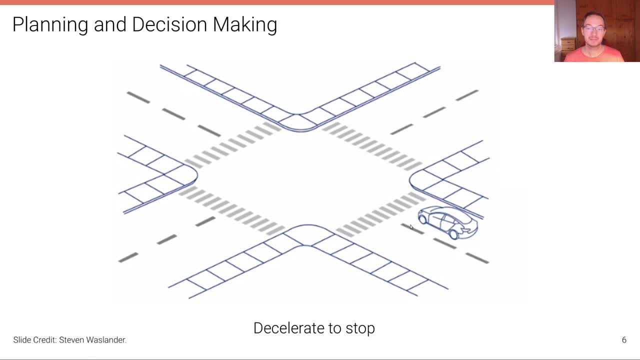 Another situation might be one where it has to stop, It needs to decelerate in order to come to a stop because it arrives at an intersection. There could also be traffic lights at that intersection and the traffic lights could be red, So in that case the vehicle needs to stay stopped and observe the traffic light in order. 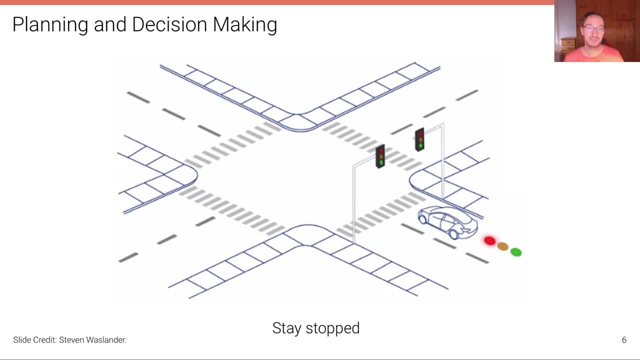 to determine when it may be allowed to start driving again, And then finally, once the traffic light turns green, it starts driving. It could also be that there's no traffic lights, but there's just a yield sign at this intersection, so the vehicle needs to observe the vehicles and other traffic participants surrounding. 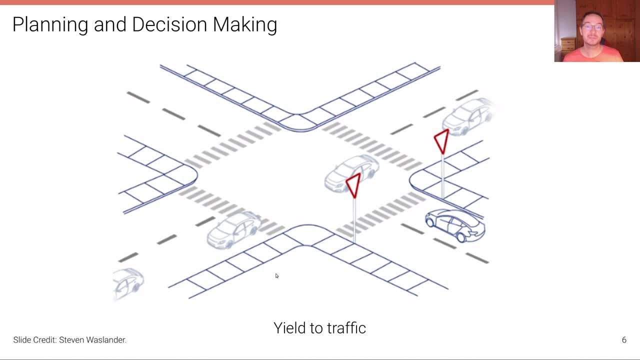 it and yield to the oncoming traffic. It could also happen that there is an obstacle in front of the vehicle or an emergency is happening and the vehicle needs to come to a full stop as quickly as possible. This is just a small set of all the possible situations that a vehicle could be in. 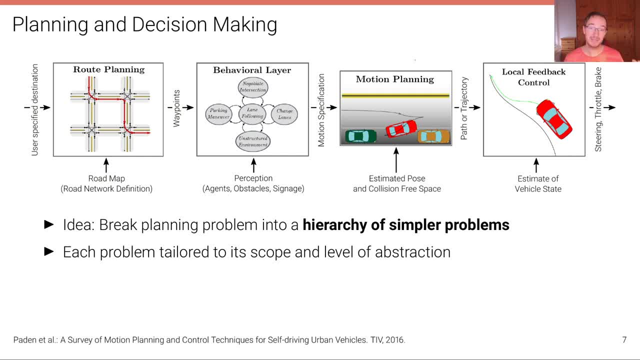 There might be many, many more, And so, therefore, the idea is to not model the entire block of decision-making and planning as a single one, but instead to break this planning problem down into a hierarchy of simpler problems, as illustrated here. 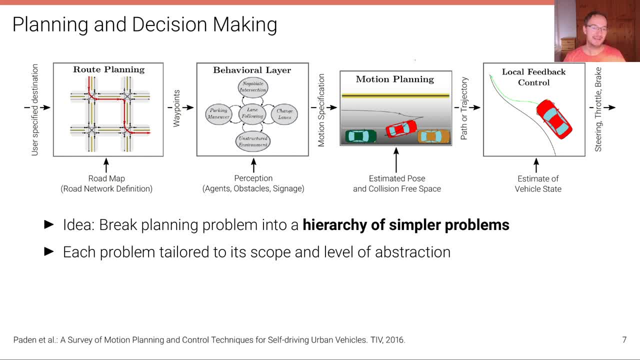 Where each problem is tailored to its scope and level of abstraction, And earlier in this hierarchy here on the left, this means we are at a higher level of abstraction. For example, in this route planning stage we want to find the approximate route from. 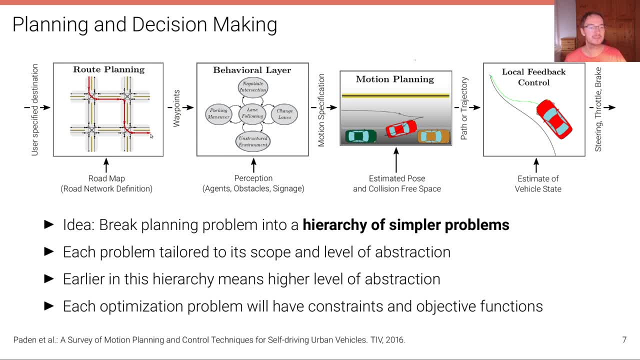 the current location of the vehicle to the destination, for example through such a HD map as illustrated here, And at a lower level, For example, here in the motion planning stage, we're trying to plan at a much more fine granular resolution the trajectory or path of the vehicle in order to perform a 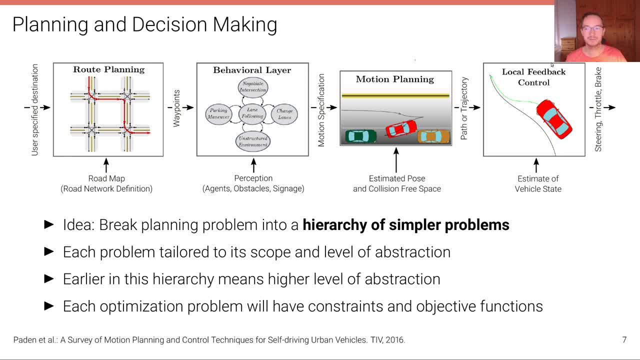 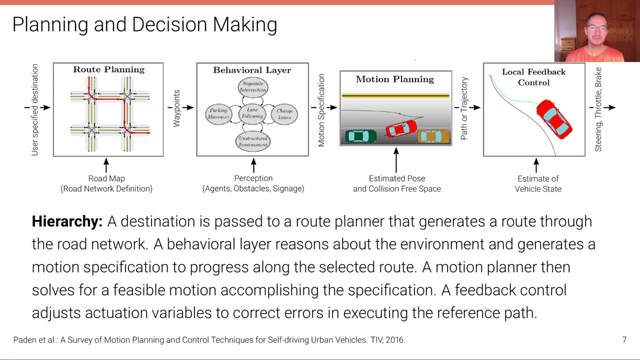 certain maneuver And that path or trajectory is then fed into the local feedback control. Each of these optimization problems that we're going to formulate here will have its own unique constraints and objective functions, as we'll see. So let's have a little bit more detailed. look at this hierarchy. 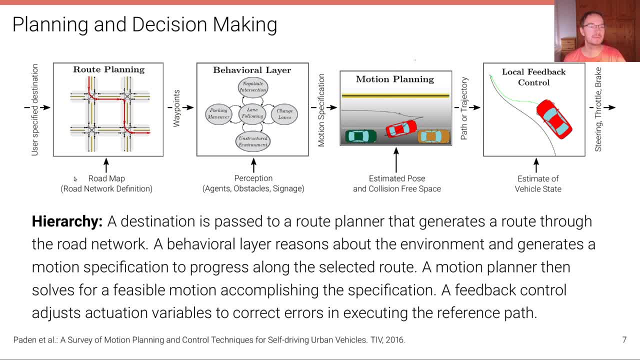 What's happening here? Well, let's start from the left, from the most abstract, the highest level. First, a user-specified destination is passed to a route planner, And the route planner is a map that generates a route through the road network. similar. 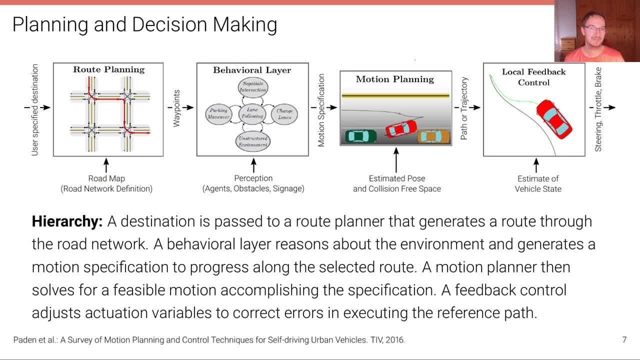 to a GPS navigation system that you have in your vehicle, but at a more fine-grained level, because it has an HD map. so it knows also lane level information. So your GPS system typically doesn't know where exactly you're located on the lane. 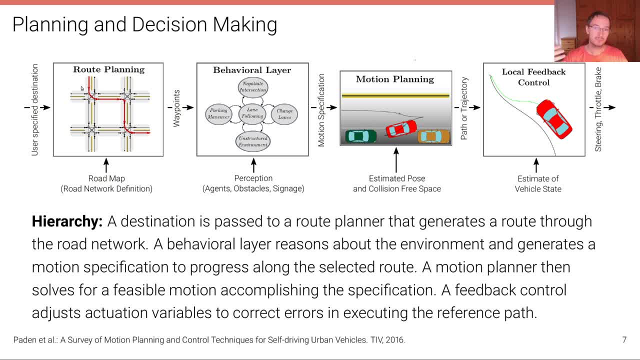 But if you have a good localization, you know And you have a good map where the lanes are marked, You know where you are on the lane, so you can map at the lane level, at lane level precision. But still it's relatively coarse, so you're trying to find a few waypoints along this. 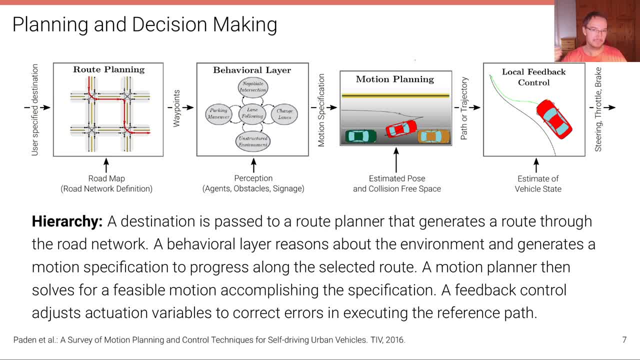 map through the city, similar to a Google Maps-like GPS navigation system. So this route planner then generates some waypoints along the road network. And you can see that the route planner generates some waypoints along the road network, similar to a GPS navigation system. 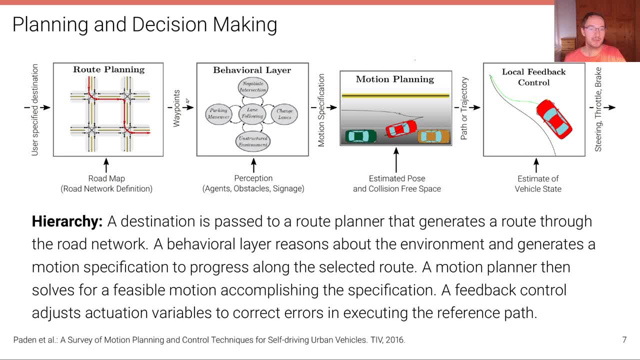 But still it's relatively coarse. so you're trying to find a few waypoints along this route that the vehicle should follow, And these waypoints are passed to a behavior layer that reasons about the environment and generates a motion specification here on the right to progress along the selected. 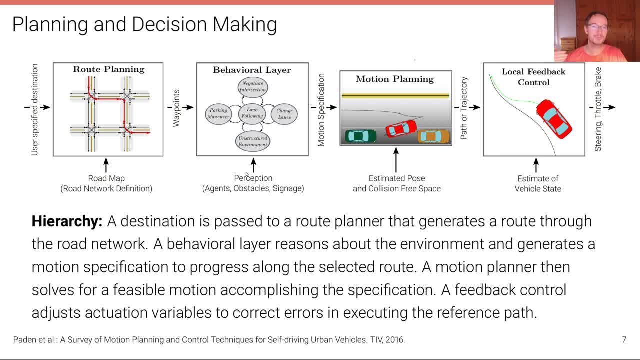 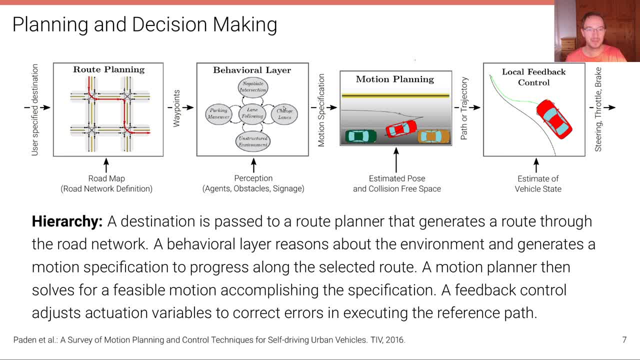 For example, information about the average day, And it can also be used to assess the conditions in the scene, the obstacles or the signage. And it can also be used to assess the conditions in the scene, the obstacles or the signage, And such a behavioral layer is typically implemented using a finite-state machine. 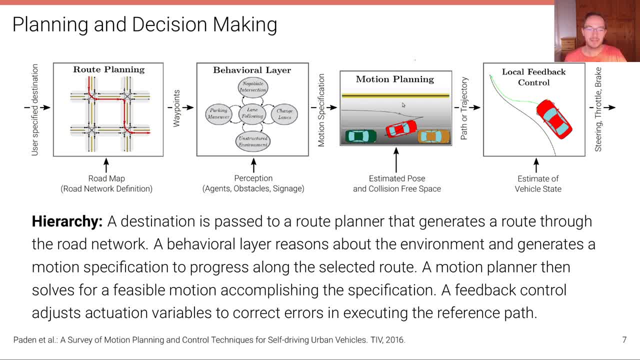 And then here we have the motion specification, which goes into the motion planner, that then solves for a feasible motion that is accomplishing the motion specification from the behavioral layer. And finally this And finally, this resulting path or trajectory is then fed into a local feedback control that 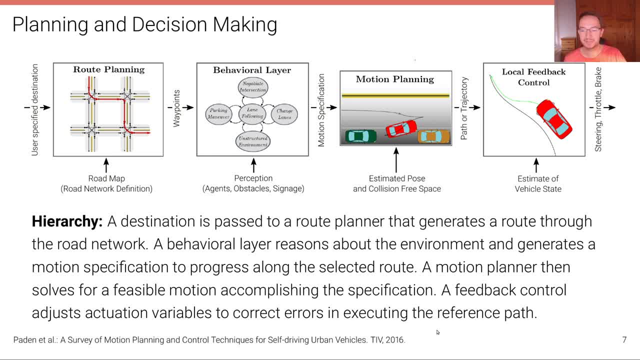 adjusts the activation variables to correct errors in the executing the reference path, so it tries to adjust steering, throttle and brake, and it obtains the estimate of the vehicle states in order to perform the local feedback control. let's now look into each of these blocks in a little bit. 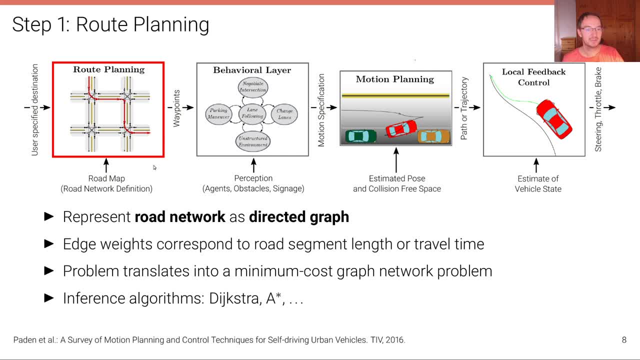 more detail. the first step is route planning. here we typically represent the road network, as you can see here, also as a directed graph that comprises notes and edges- directed edges- with these little errors you see the direction here- that connect these notes and that indicate along which paths the vehicle is allowed to drive. typically this: 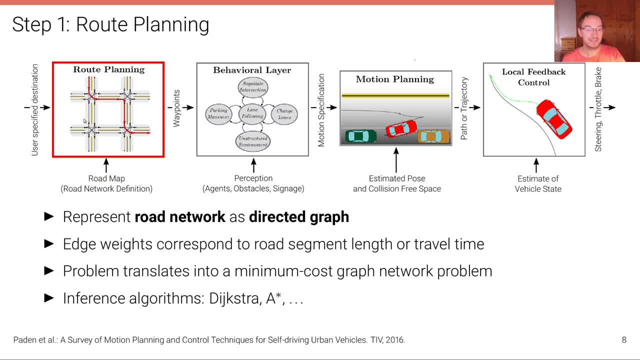 directed graph is a weighted directed graph where the edge weights correspond to road segment length or travel time that can be taken into account by the inference algorithm for finding the most efficient route to the destination. this problem is then translated into a minimum cost graph network problem that can be solved using standard. 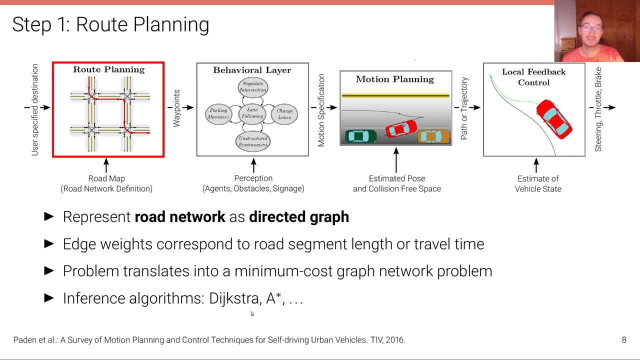 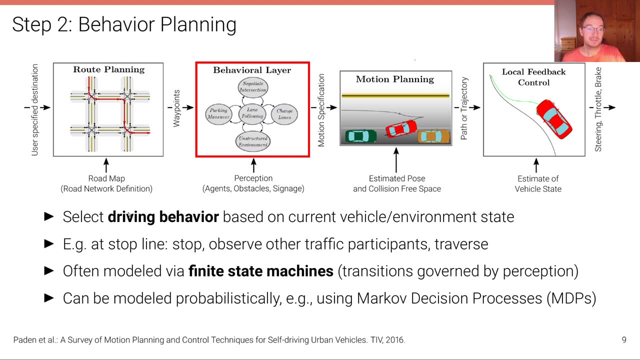 inference algorithms from the graph literature, such as Dijkstra or ASTAR algorithm, and we'll look at these algorithms today as well. the second step is the behavioral layer. the behavioral layer selects a driving behavior based on the current vehicle or environment state. example, at a stop line it stops. next it observes the other traffic participants. 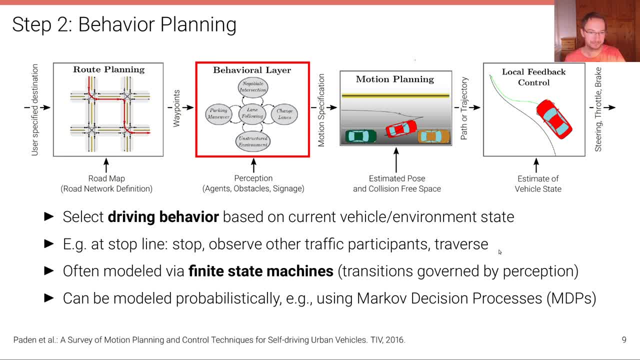 and finally it traverses the intersection. the behavior layer is often modeled using a finite state machine, or FSM in short, where the transitions are governed by perception, but it can also be modeled probabilistically, for example using a Markov decision process that we've already seen in early lectures. the 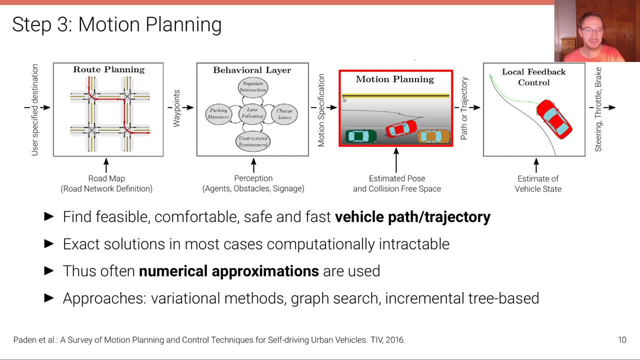 third stage then is the motion planning stage. that takes in the motion specification and produces a path or trajectory. so the goal of the motion planning stage is to find feasible find a feasible, comfortable, safe and fast vehicle path or trajectory based on the motion specification, the, the. the computation of the exact solution is, in most cases, computationally. 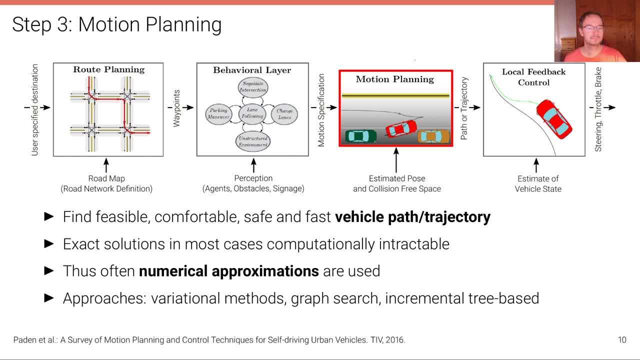 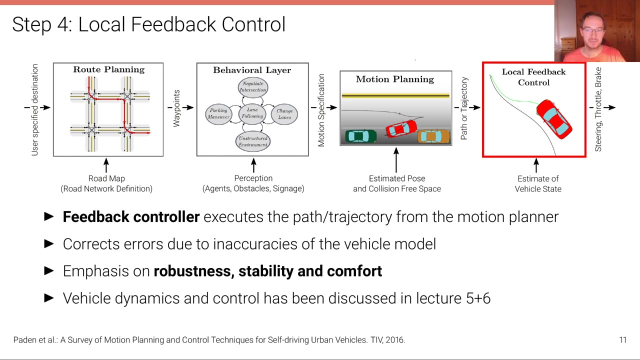 intractable, and so therefore, often numerical approximations are used, and typical approaches- that we'll briefly discuss- for solving the motion planning problem are variational methods, graph search methods or incremental tree based methods, and then, finally, we have the local feedback control that takes in the 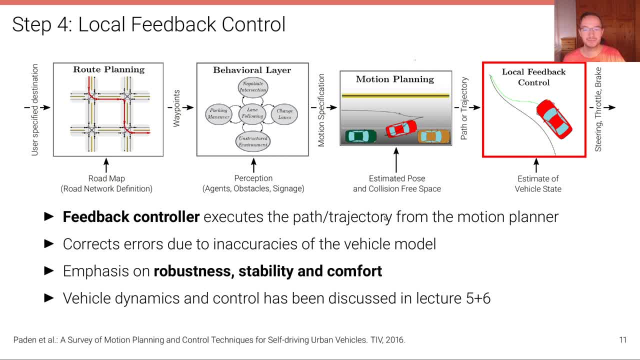 path or trajectory from the motion planning stage and executes it, and it executes it such that it corrects errors due to the inaccuracy of the vehicle models, just as we've seen in the lecture on vehicle control. the emphasis during control is, of course, on robustness, stability and comfort, and most of our vehicles already are equipped.